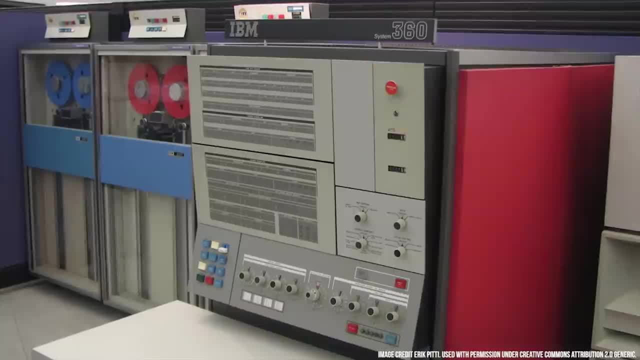 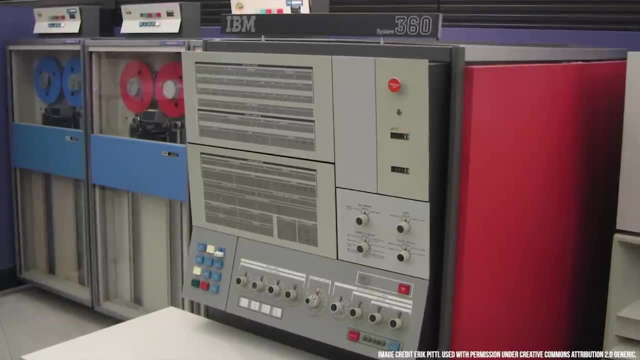 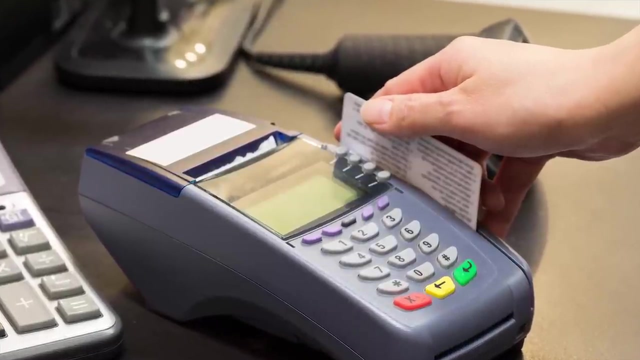 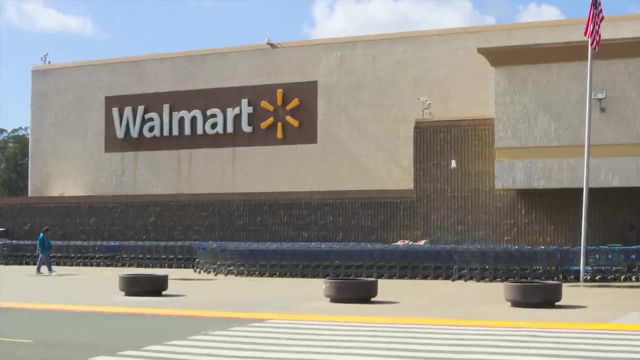 simpler transactions extremely quickly. In fact, even though there is a popular misconception that mainframes are relics of a bygone computing era, to process the up to millions of card swipes and account transfers that occur daily, 96 out of the world's top 100 banks and 23 out of the top 25 US retailers currently run mainframes from IBM. 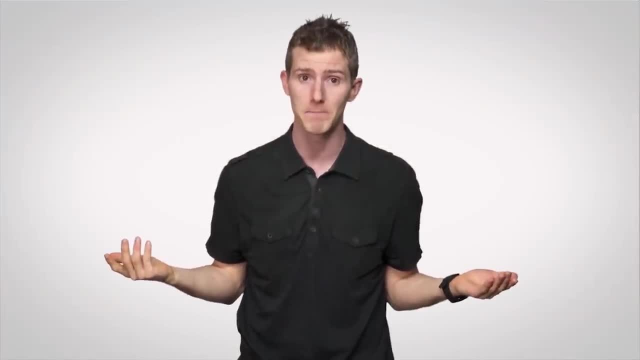 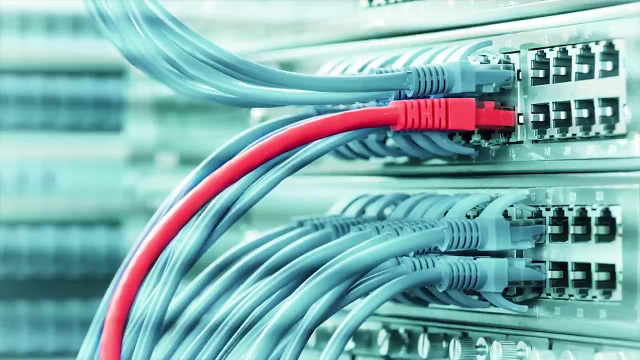 who has been the dominant player in the industry for a very long time. Building one, though, isn't just a matter of installing a whack ton of Xeons in a box, plugging in lots of ethernet cables and calling it a day. 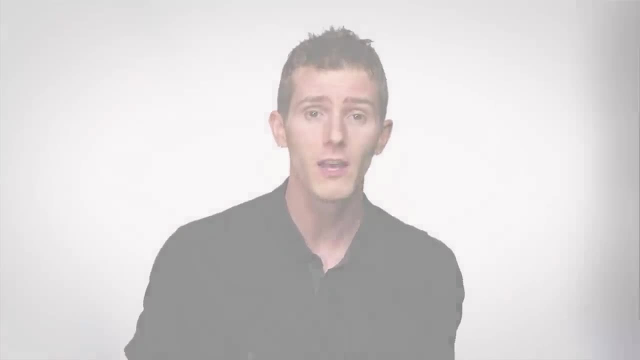 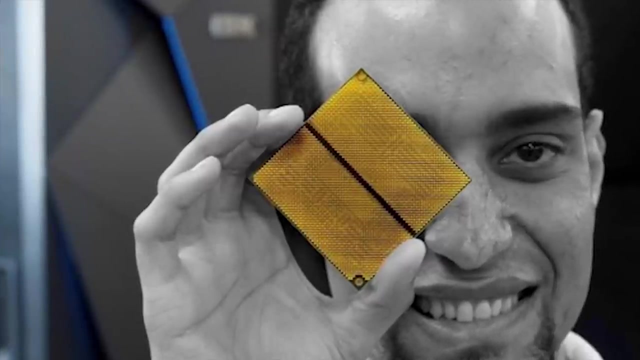 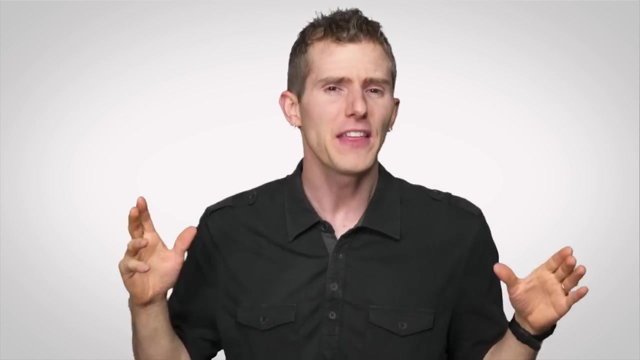 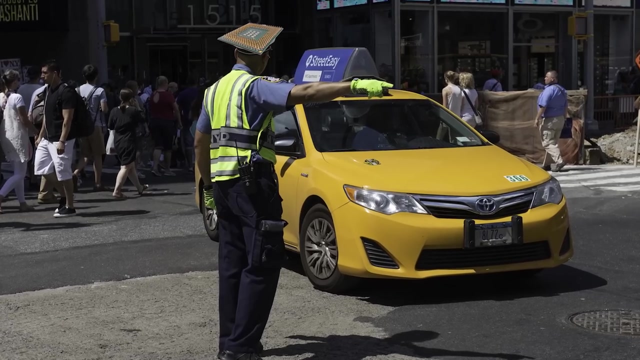 Mainframes use special CPUs, many of which are much larger physically than even big desktop chips like 2011 socket CPUs from Intel, as well as additional processors called System Assistance Processors or SAPs, that do almost nothing but move data around as quickly as possible like glorified traffic. 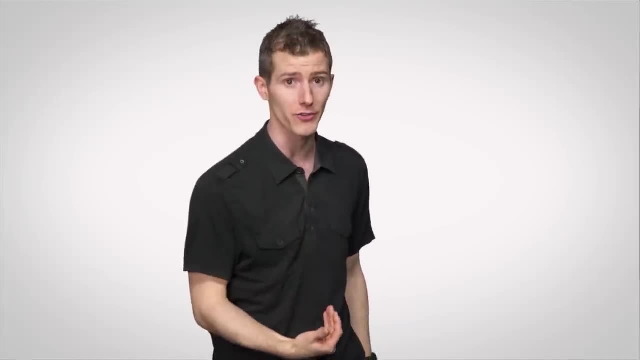 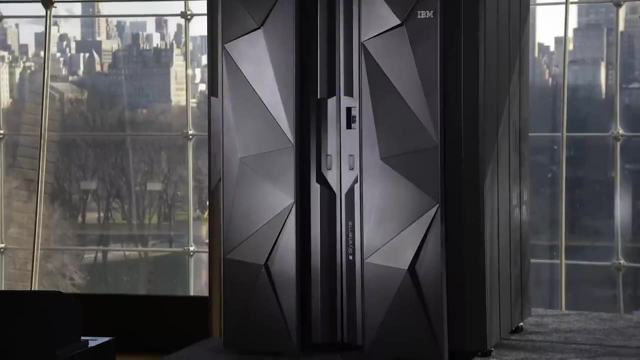 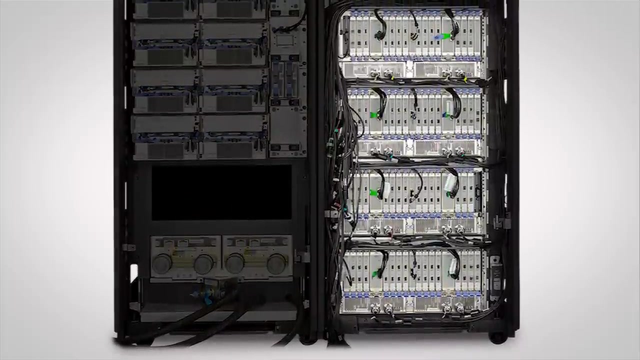 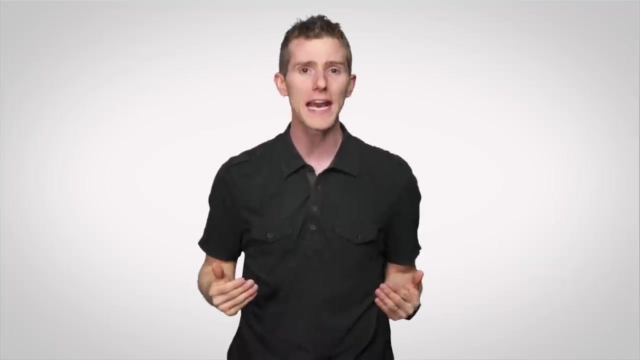 controllers rather than general purpose number crunchers. And that's not all. On a modern mainframe like the top-end IBM Z13,, each individual IO card- of which there can be 160, has its own processing cores, up to two per channel on the dual-channel cards, meaning you could have 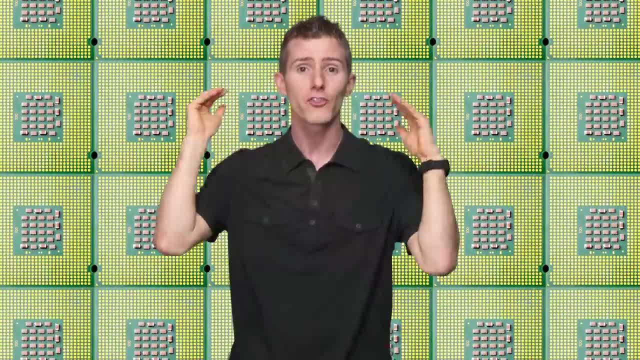 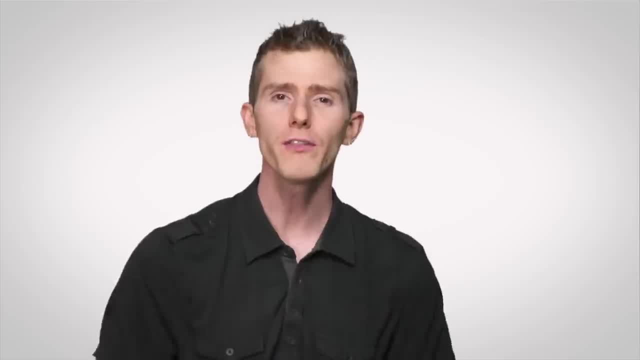 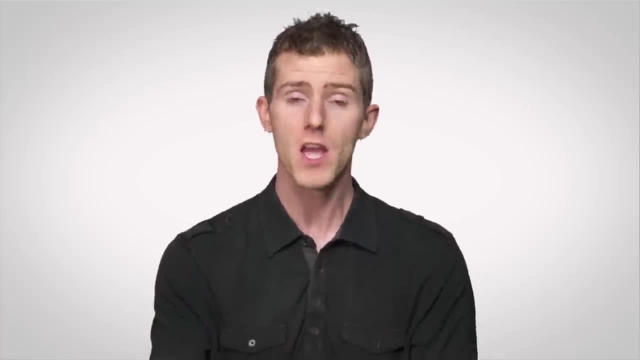 over 600 processor cores just for IO, and that's not even counting the SAPs. Whoa. Part of the reason that modern mainframes are designed to support this many IO is to ensure that they stay reliable. so many of the subsystems inside a mainframe, like a modern airliner, would. 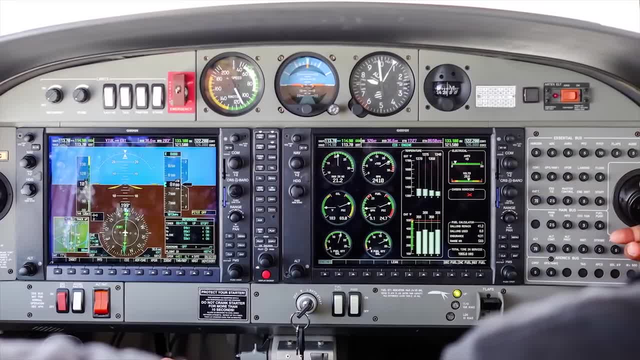 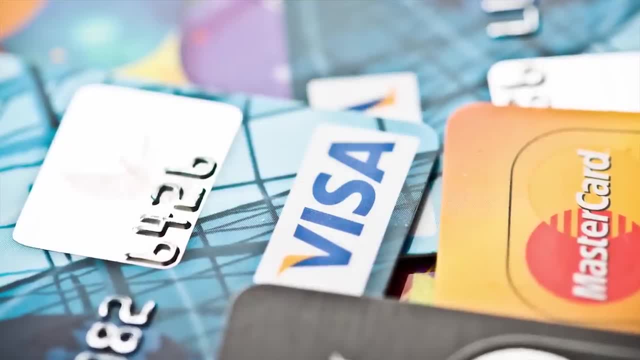 have redundancies built-in. This means they can be deployed in situations where zero downtime is acceptable, such as the aforementioned credit card companies and retailers, as well as airline ticketing systems. In fact, a common mainframe counts low, so it's действований streamlines low for about 30 minutes. 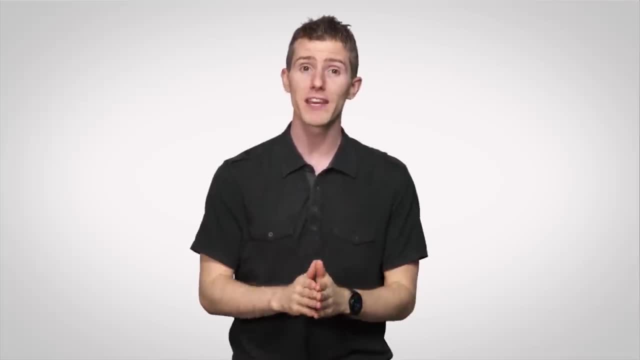 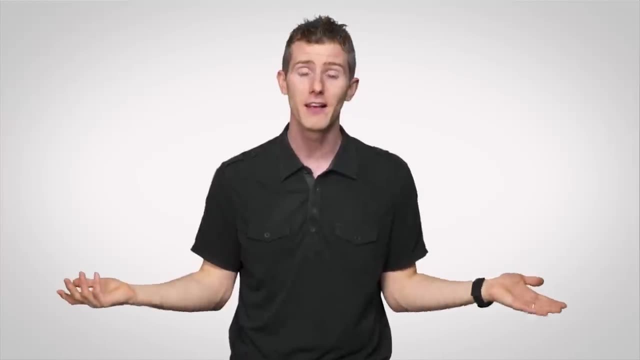 up to 60 FPS in a patients room, compliant to schedule, officials and customer activity. there still has to be a betaiche running persona operating system. IBM's proprietary ZTPF was originally developed as transaction processing software for airlines. If you want to see it in action, pay close. 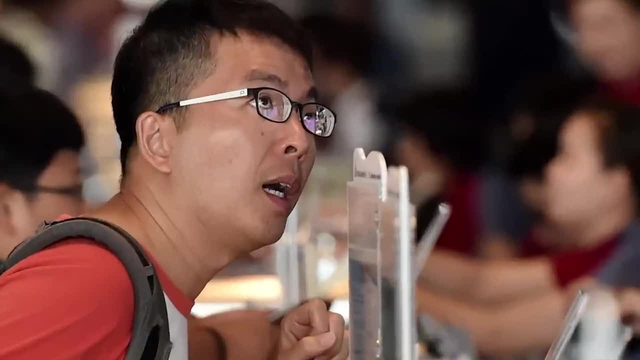 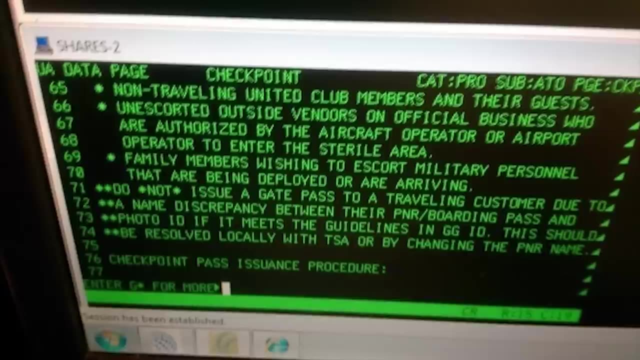 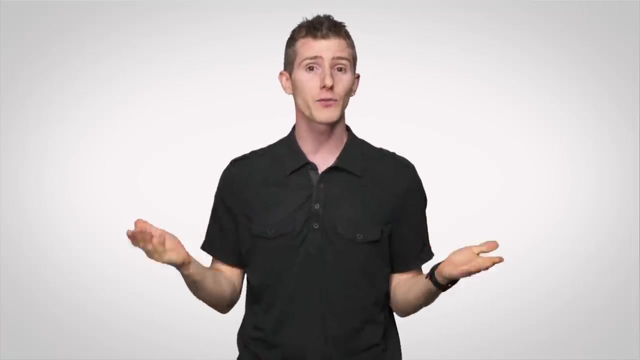 attention next time you board a flight and you might just get a glimpse of the computer screen they're using to check you in. An old-school interface with green text indicates that it's probably a terminal connected to a mainframe. Just don't look too closely at it. So this high level of redundancy means that it's 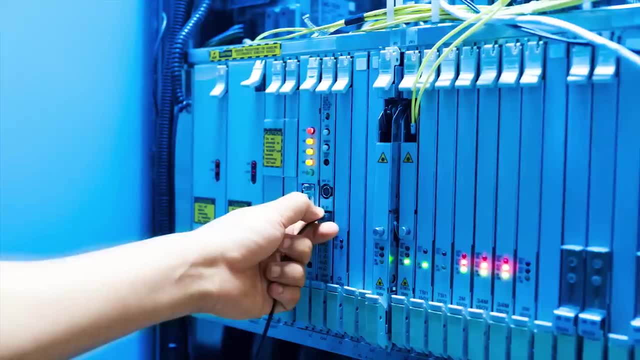 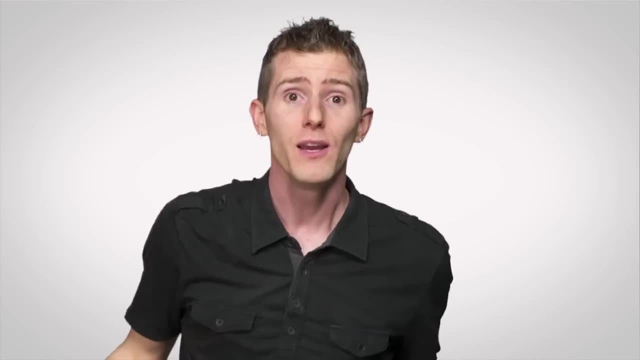 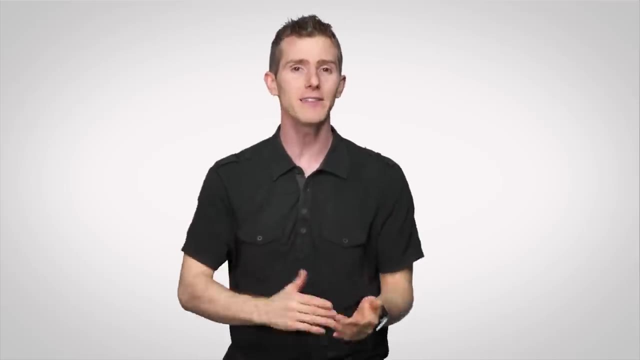 common for mainframes to be built in such a way where an administrator can slide out one of the drawers that houses components and simply start swapping them out. Whatever that drawer was working on is automatically transferred over to the rest of the mainframe, making it easy to make necessary hardware. changes without any downtime, Which is a good thing too, because high-end mainframes don't have to be built in such a way that they can be easily managed. A single mainframe can run tons of virtual servers at once, up to 8,000 in. 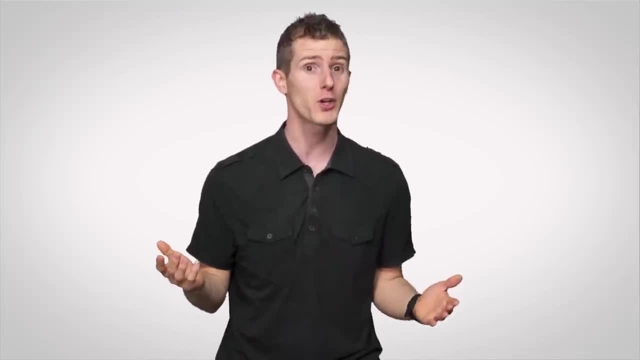 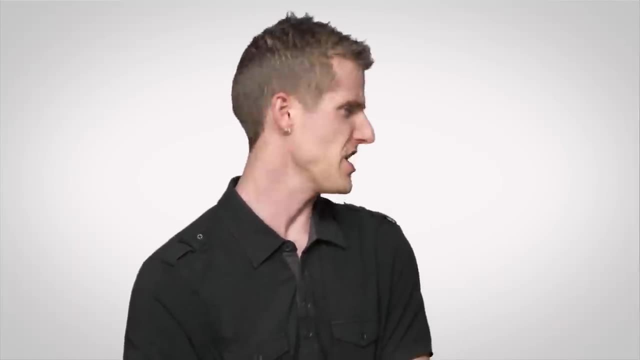 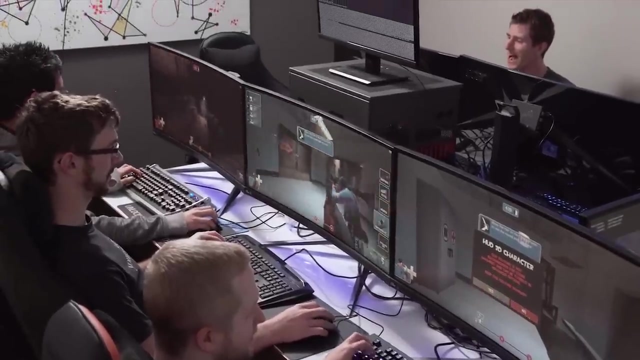 the case of the Z13, meaning that taking down the mainframe could result in a lot of transaction errors on Black Friday. But before you start thinking, gee, I should get myself a mainframe because I want to run Overwatch on like some kind of 50 monitor setup. mainframes and their operating systems aren't just absurdly. 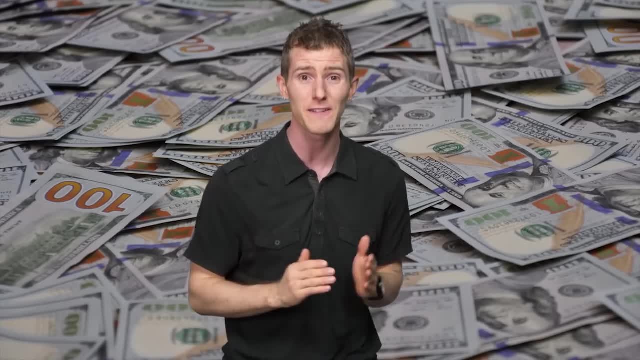 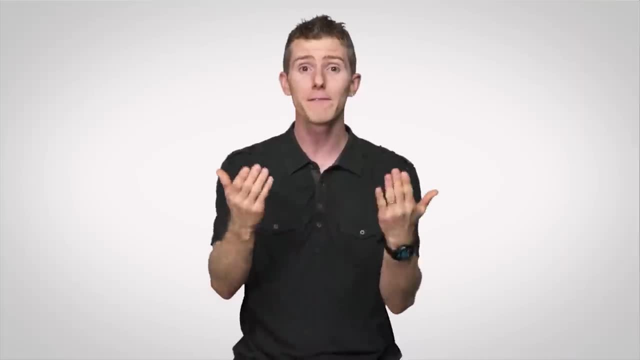 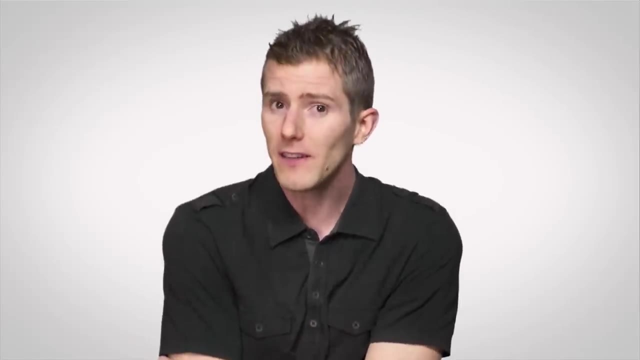 expensive. A single mainframe can cost hundreds of thousands, if not millions, of dollars. They also aren't designed to run games or for high-end floating-point performance, which is important for rendering graphics. But even so, mainframes are still in the background, powering lots of. 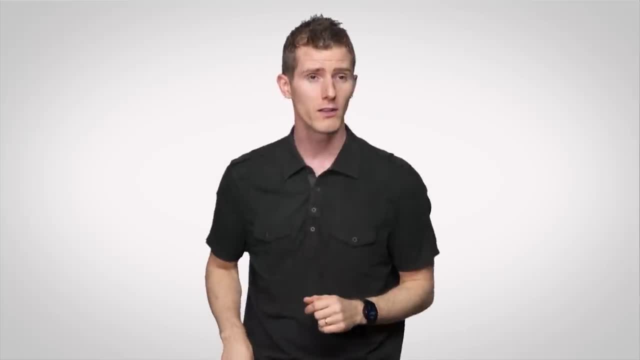 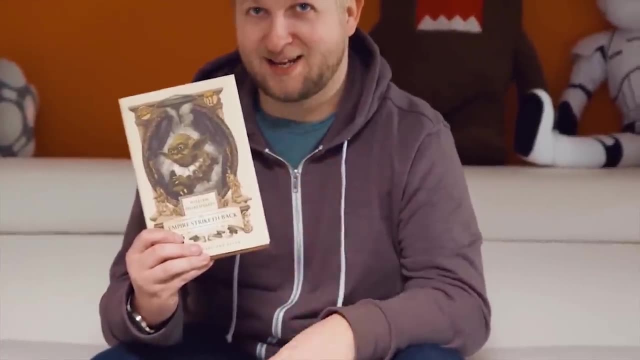 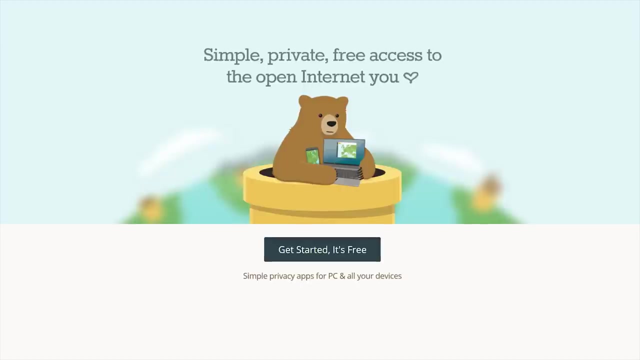 things you do every day, which is pretty cool, That is, unless you've sworn off air travel and you don't want MasterCard to know about all the weird stuff you buy on Amazon. Speaking of having your online activities tracked, TunnelBear VPN lets you anonymize yourself on the internet and browse the internet. 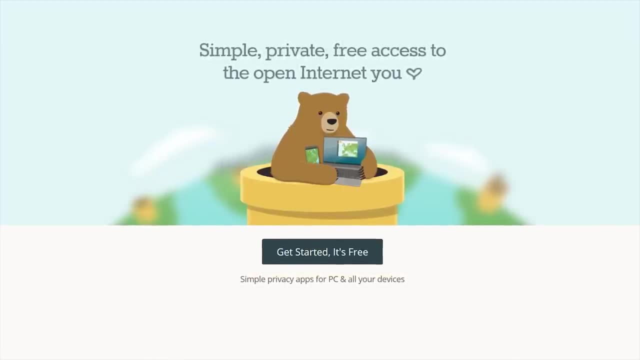 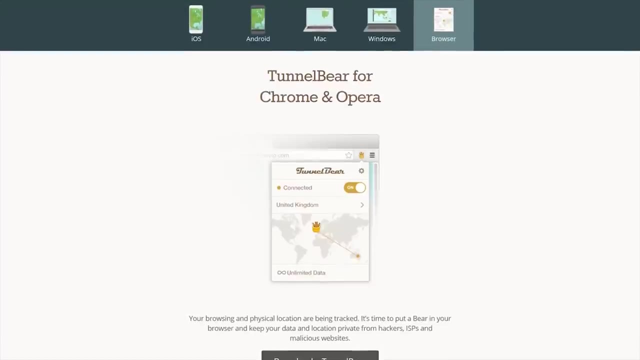 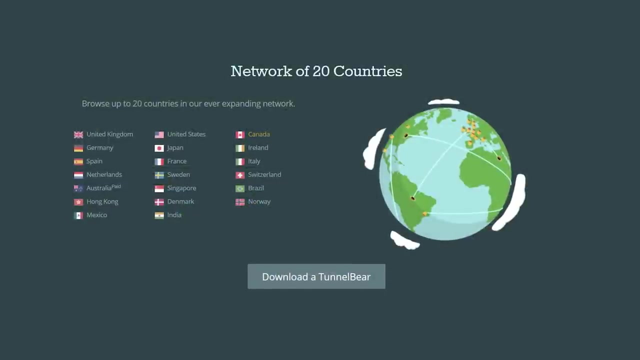 and use online services as though you are some anonymous guy in some other country. They have easy-to-use apps for iOS, Android, PC and Mac. They also have a Chrome extension and it's super easy to use. You just press a button and boom- TunnelBear is on Your. 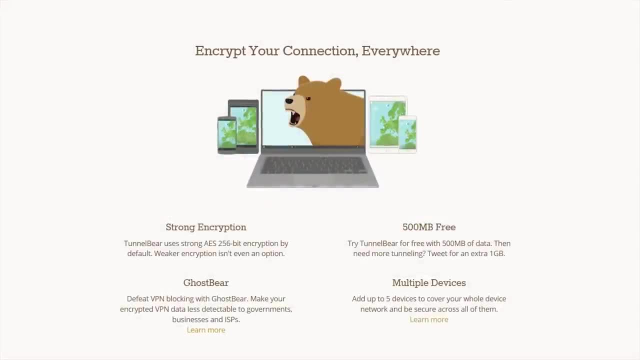 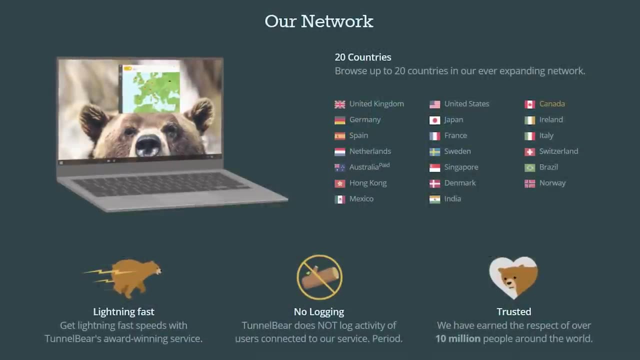 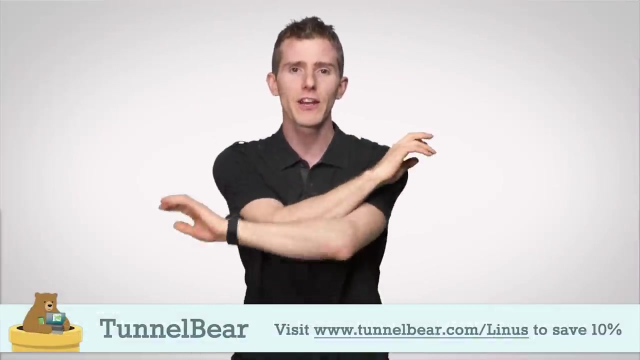 connection gets encrypted with AES 256-bit encryption, and your public IP address gets switched, So you show up as though you are in a different country. TunnelBear makes it easy by bypassing all the annoying details that typically come with using a VPN: No DNS, no router configuration, no port configurations- none of that nonsense.